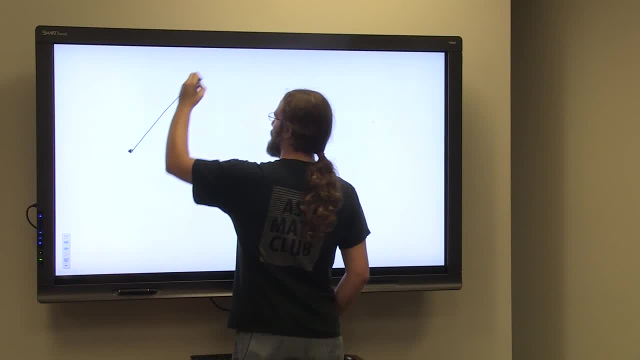 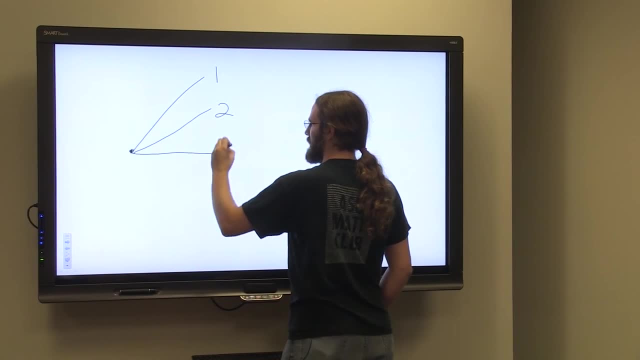 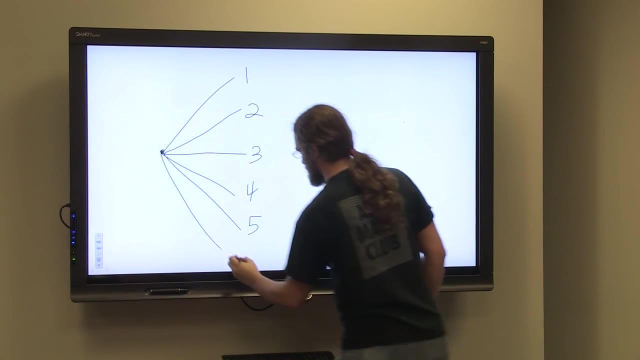 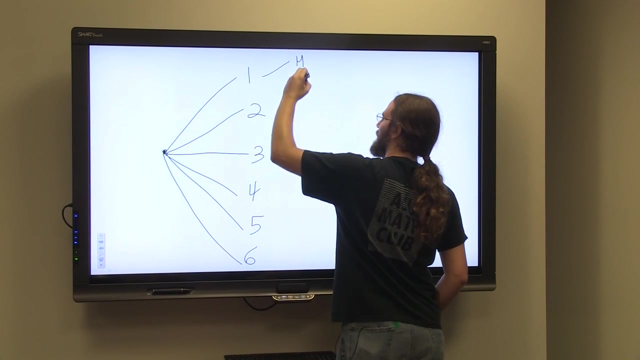 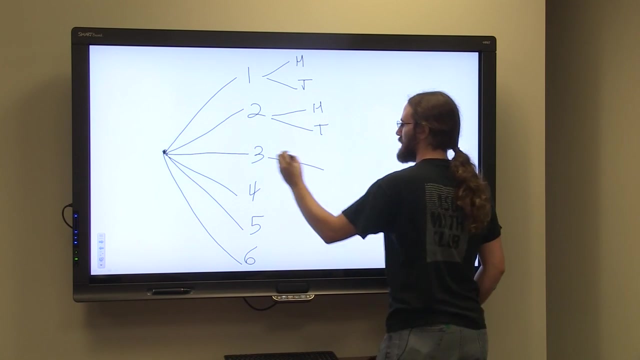 by rolling our die. We can roll the die and get a one, a two, a three, a four, a five or a six. We can flip heads or tails, heads or tails and so on. My diagram here might not be the. 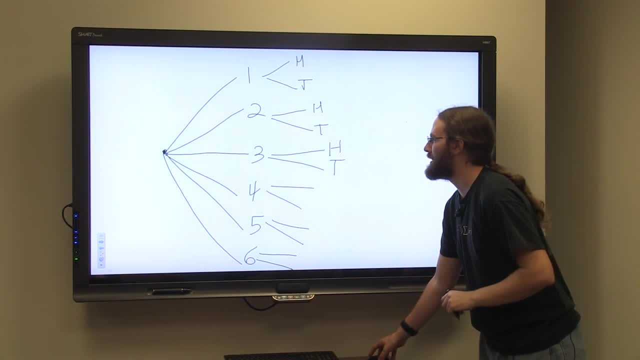 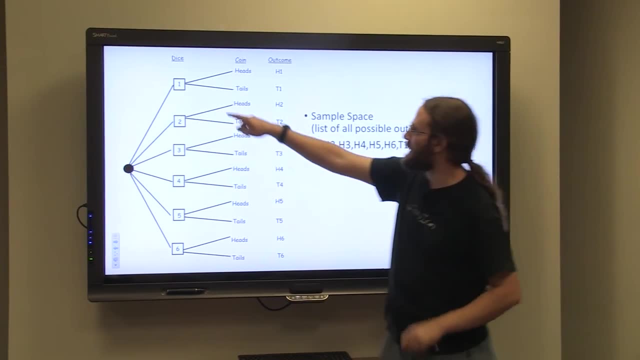 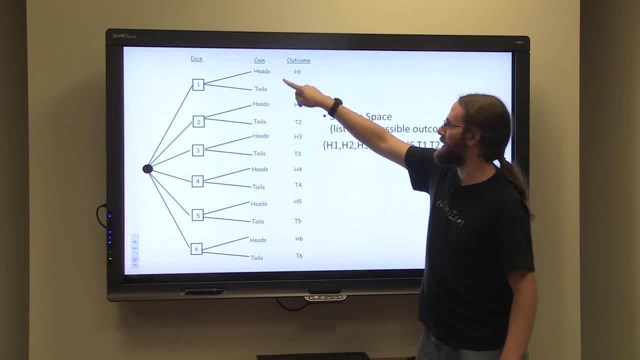 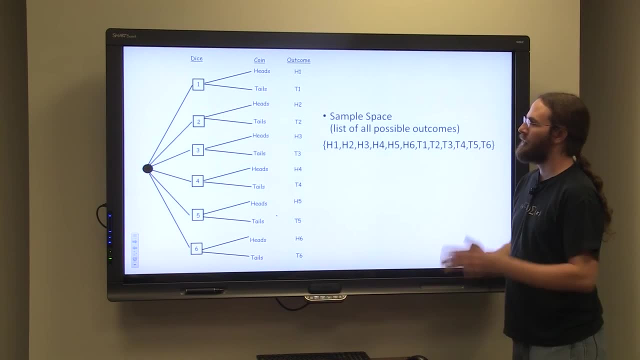 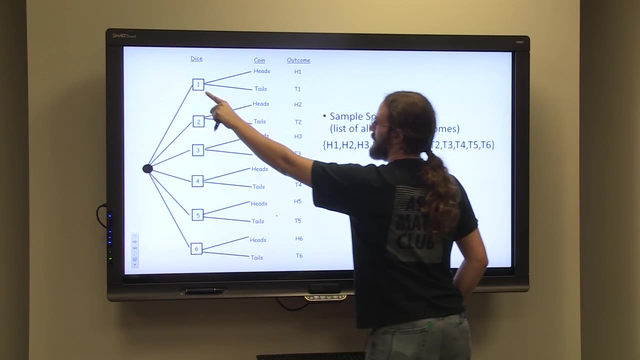 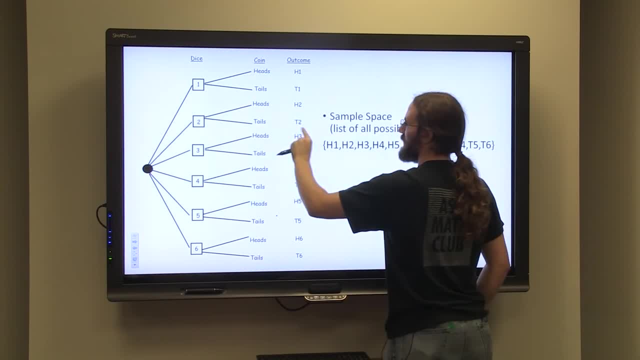 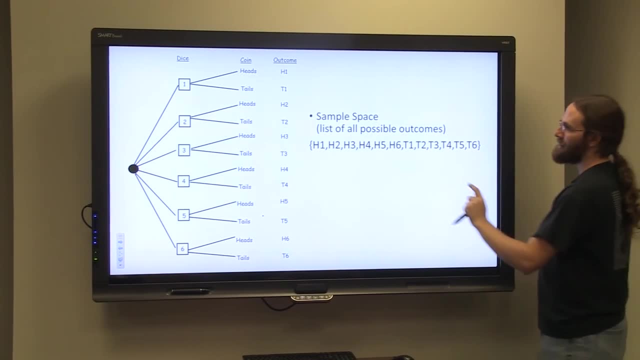 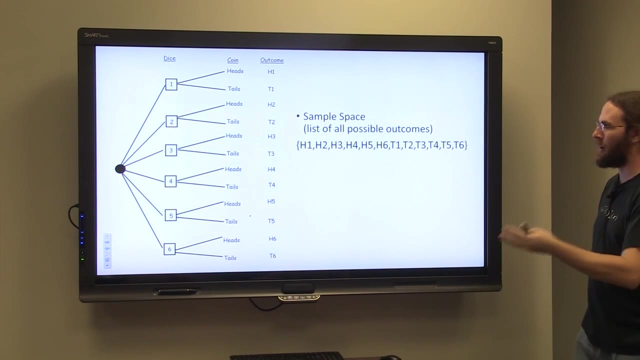 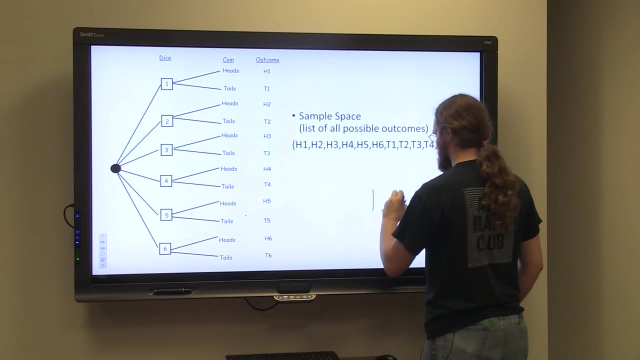 flip tails and a 1, so on and so forth. So I have all 12 outcomes listed here and I decided to go ahead and list them out here in what we call a sample space. A sample space is simply a listing of all possible outcomes, So you can count up here. there are 12 outcomes. 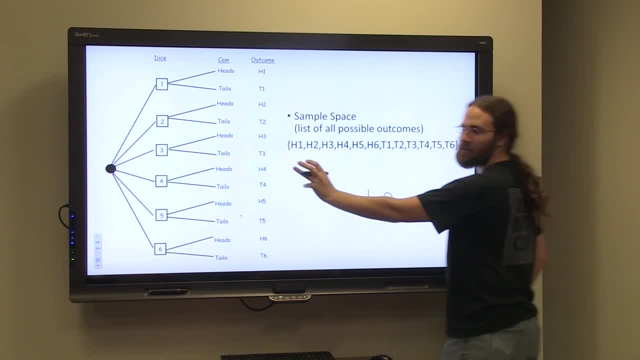 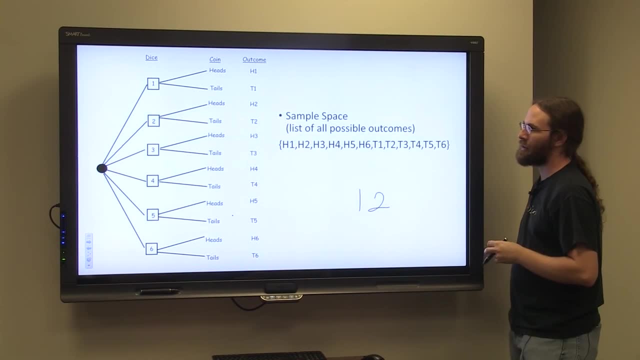 Drawing a diagram is fine, but sometimes drawing the diagram can become cumbersome. It can become labor intensive. When we start looking at, perhaps, rolling a dice four times, or rolling four dice, or perhaps flipping a coin 20 times, drawing a diagram can become very cumbersome. 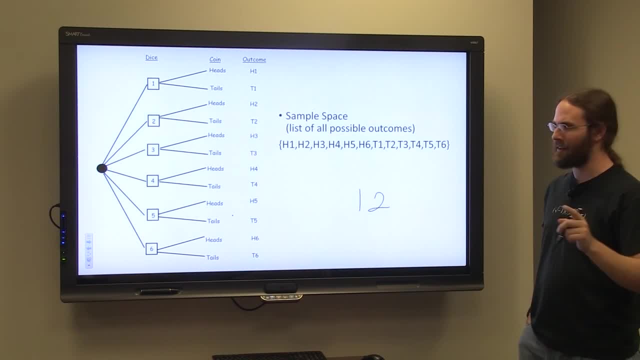 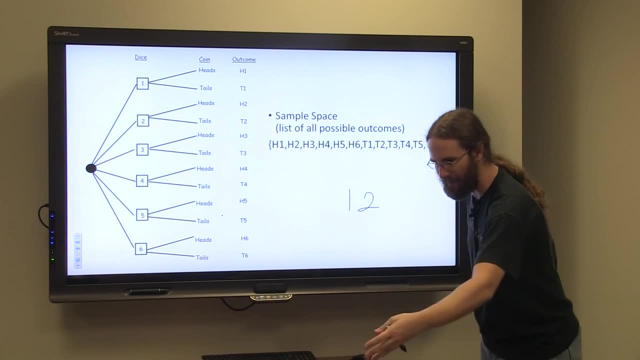 So first let's talk about: is this an independent event? As in, when I flip a coin, does it care what happened with my die? Does the coin care that I just rolled a 2? Or does I just roll a 3?? When the coin is in the air, is it thinking?